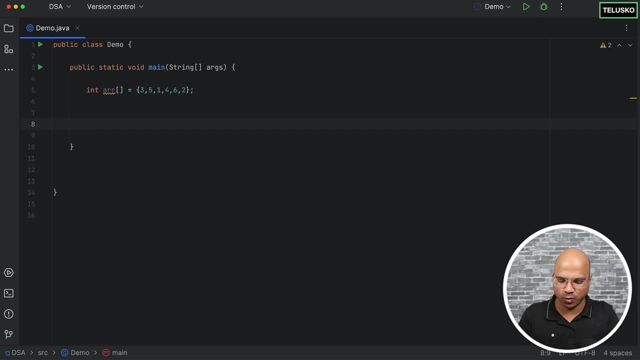 here And let's apply the sorting techniques on this. So before sorting I will print some values. I'll say for in n in array And let's print this values. So I will say print n. but I will also make sure that I will put a space. I will not print on new line And 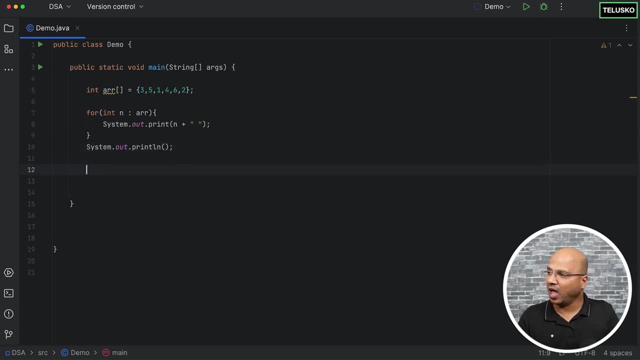 once it is done, I'll print on print a new line And then after sorting also. so I will say this, I will just write it here after sorting. So here, let's, let's do the same thing And let's after sorting, it should print some value. But at this point, if you 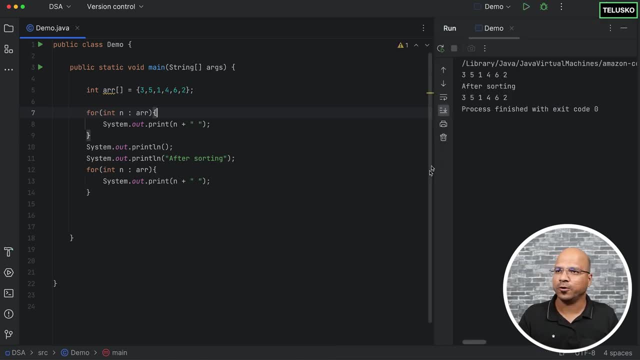 run this code, let's run this And you can see in the output they both are unsorted. So, because that's why we have to do some sorting here, right? So let's apply the sorting logic. So what I will do is I will simply call a merge sort method, which will basically accept three. 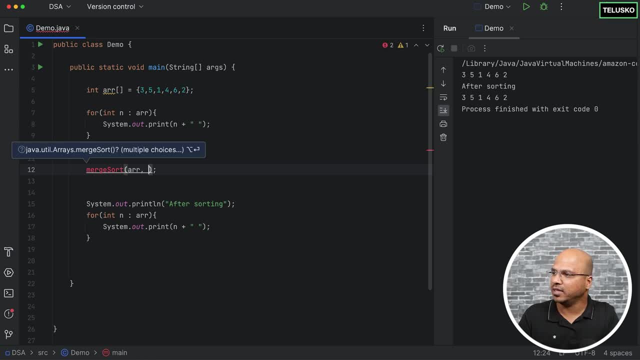 values, the ARR, the L- now L here is zero. And then you have to also pass the array dot length minus one, basically have to pass the R value as well. Remember, we have to pass three variables. Now, since we don't have this method, I will simply say: more action. 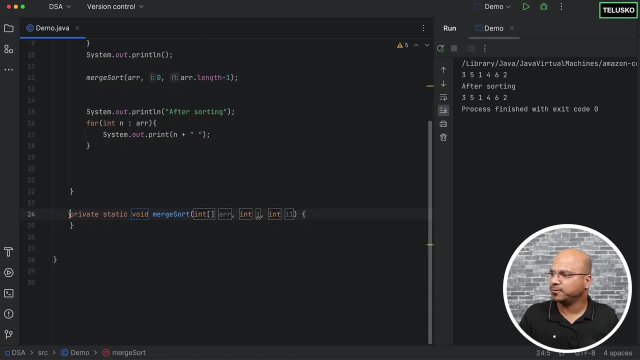 here. So let's create this method. And you can see we got this method here. And let me just put this method not here, but on top. Now this is where the actual logic is going to happen. So you can see, we got two variables: this should be L and this should be R. So 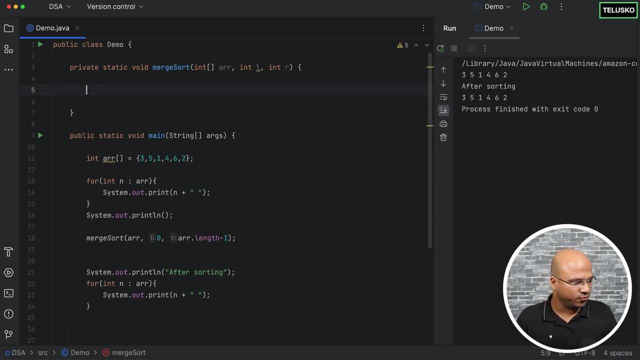 left and right. Okay, Now as for the logic, if you can see, in our logic we have already mentioned this logic. So basically, what we're to do is we have to first check if the L value is less than R, then only you do certain things, And what are the things you have to do? So 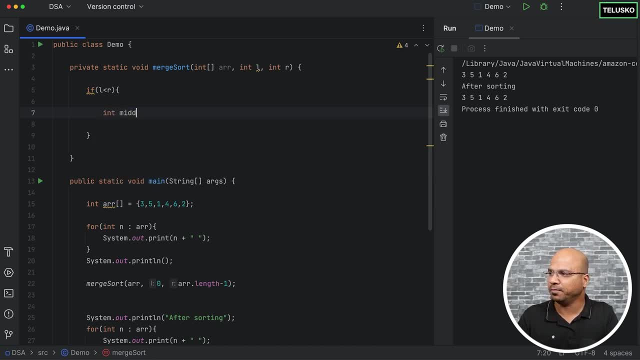 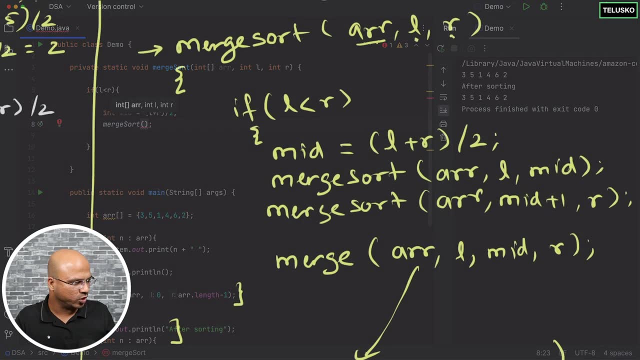 basically you have to find the middle value. So I will say int mid is equal to L plus R divided by two. And then you have to call merge sort two times Again. I'm just going with the logic which I've written in the code or in the board here. So to pass ARR and 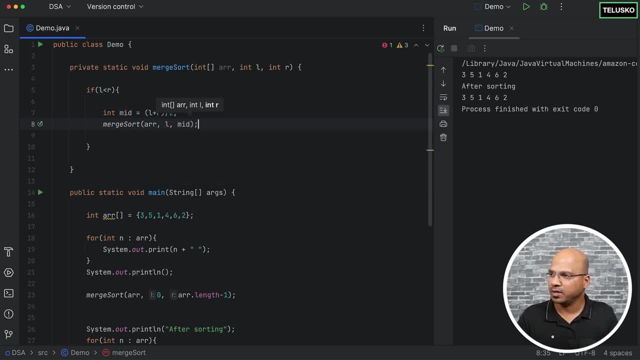 then you have to pass the L, and then you have to pass mid. That's how you create two different arrays, So mid plus one and R. Okay, and then you will simply say: merge. Of course, right after doing this, sorting, after breaking it down, you have to also merge, So you have. 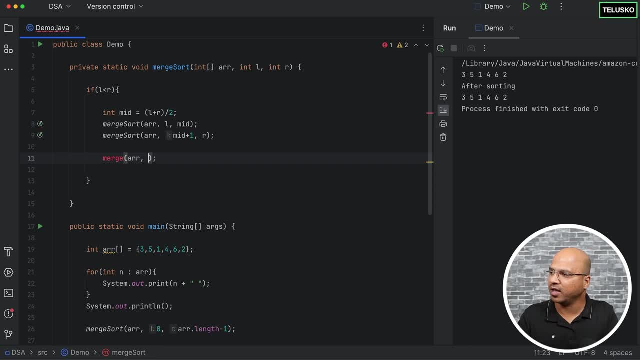 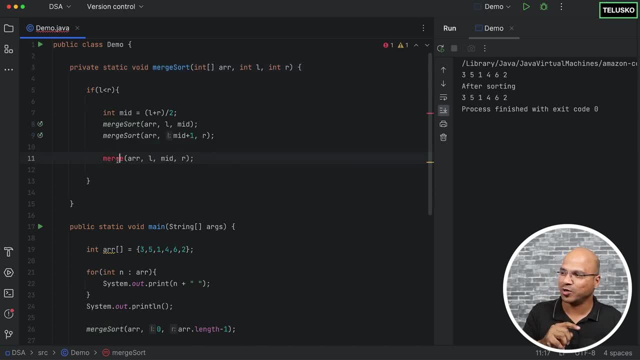 only logic. you have to write inside merge sort method, But then we have to also complete merging, because dividing is very easy. This is how, basically, you are dividing the values. The difficult part is merging them. So let's implement merge here. So I will just go back. 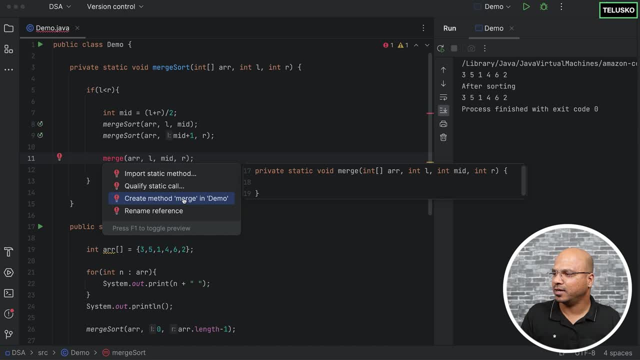 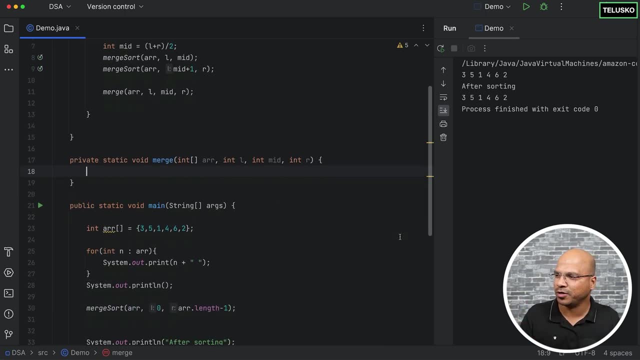 here. More actions, Create a method, merge, Yes, okay, So I got a method. At this point they are private methods just because I'm going to call from the same class, But, depending upon your requirement, you can just change them. 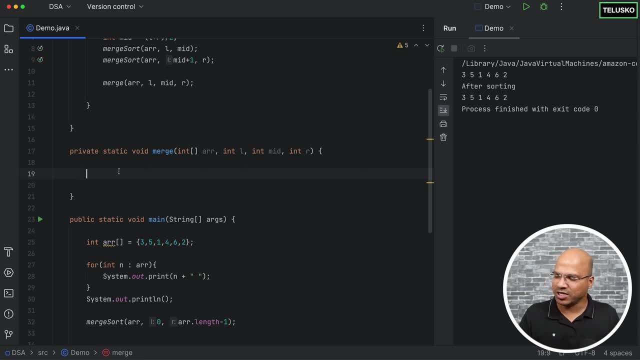 And now the actual logic goes here: the merge. Okay, now, as I mentioned, you need to create two arrays here, right? So, if you can see the logic, we need two arrays. Let's name this as LRR, which is the left array, And this will be an array. But the question is: 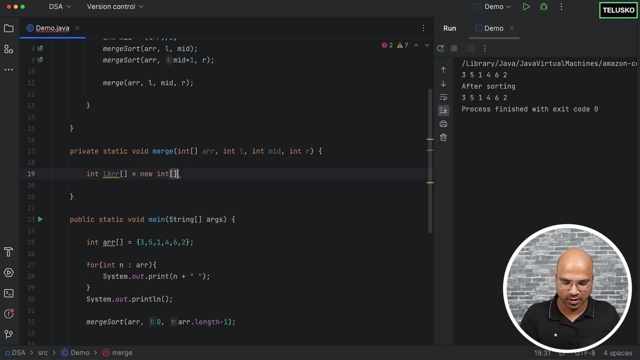 what will be the size of it? Because when I create this array, I have to mention the size. I don't know what is the size here, So I'm going to say LRR And then I'm going to change the size here. Now, based on when it is getting called, it will be different. 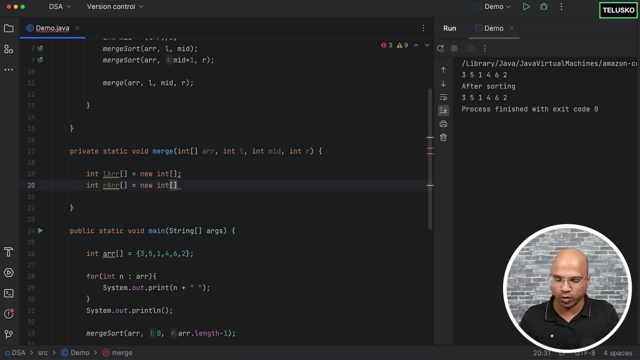 size. But the question is how we are going to know the size, And that's where this LM, all this thing comes, or LR, comes into picture. So let's use that and let's get the size. So if you want the size of the first array, the first section, basically, you can simply 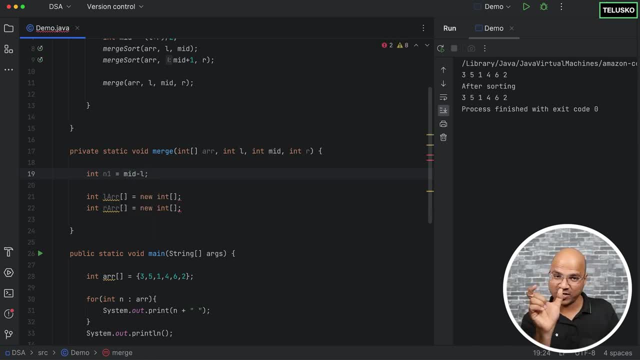 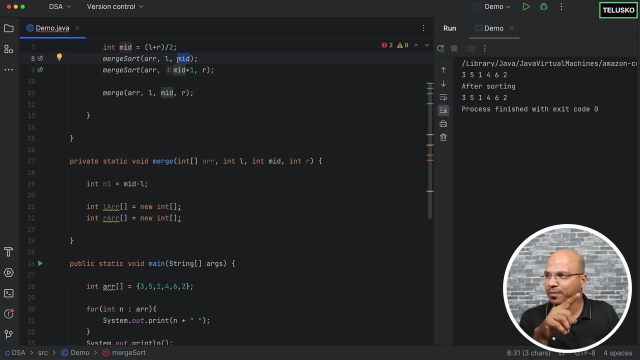 say mid minus L Because for the first array it starts with L. If you can see here it starts with L and ends with mid. So if you say mid minus L, you will get the length right. But the problem is since this: 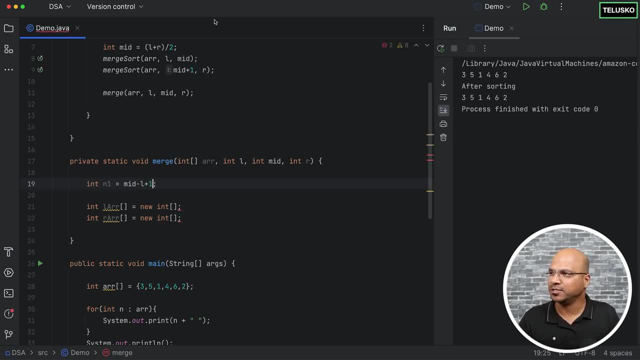 is zero indexing. we have to also add plus 1, because mid is not representing the size of the array, It represents the index value. So you have to say plus 1.. Then you will get the second array length with the help of R minus mid. So we'll just put some space here. 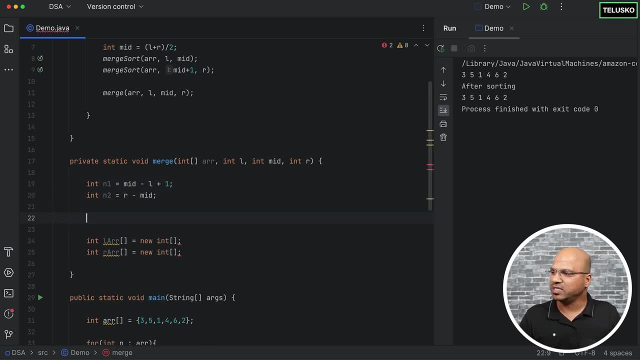 so that it will be much more visible. Okay, so you can see. we got these two values And this is the size you have to mention here. The first array will be of size N1.. The second array will be of size N2.. So it will be of size N1.. And the second array will be of size N1.. 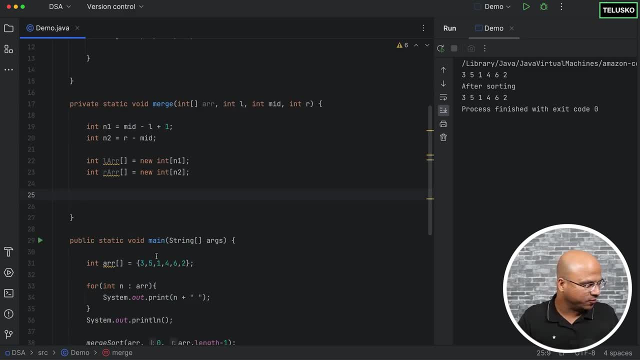 two. that's done. the next step is actually to copy the values. if you can see, we are mentioning the copy values here, right in the in the nodes. now, how do you copy value? we can use a for loop and let's use two different variables. i will say x and y this time. x is equal to zero and depend on 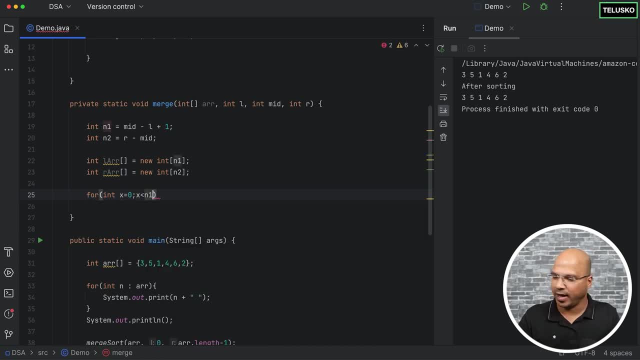 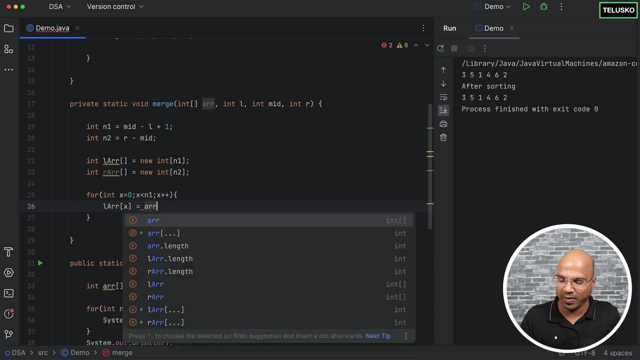 the size of the array. so for the first array the size is n1 and x plus plus. not used to using x and y inside a for loop, but let's try. so how do you copy, so arr, this values, which is x? now how will you get the values so from arr, from the main array? we have to start from the left. so i have to say: 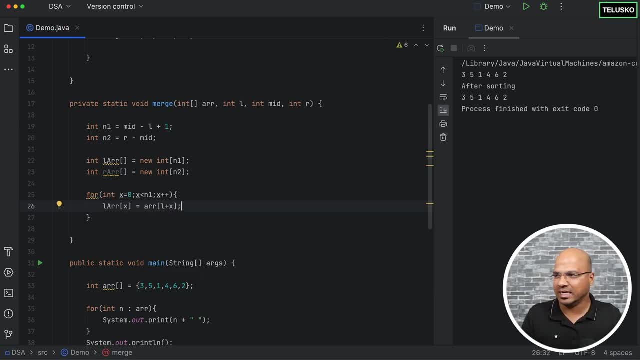 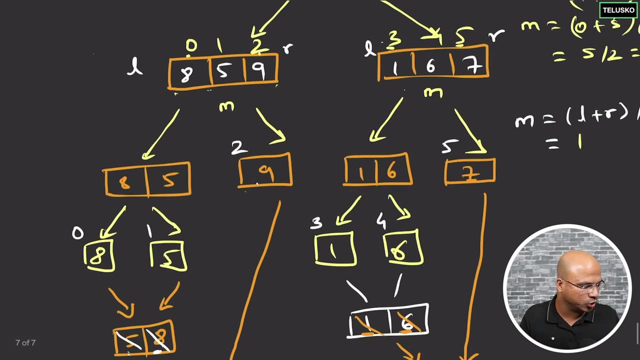 left plus x. that's how you get the values. so whatever value of the l is example, if you look at here: uh, for the first array the index is 0, 1, 2. but let's say, if you are merging the second array, this one, the index value is 3, 4, 5, right. so whatever value of 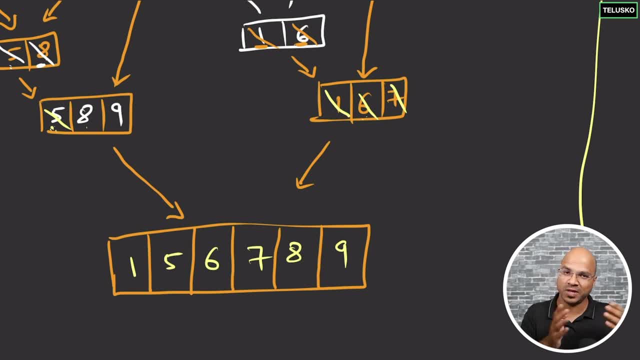 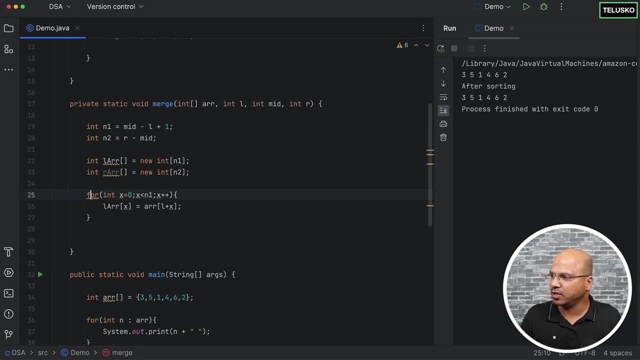 l is uh, southern is, which is the left, which is 3. in this case, it is 3 plus x. that's how you will copy and then: so this is for the first one. let's do the same thing but a different value. so I will just copy this: 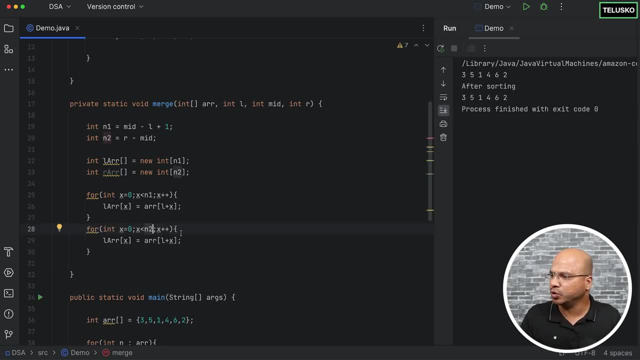 for the second array. okay, we can also use x here, no problem, we can say n2 and this will go into the right array. but the question is, what will be the value here now, any guess? so when you say on the right hand side, it is your mid plus 1, because we are not considering the mid value for the next. 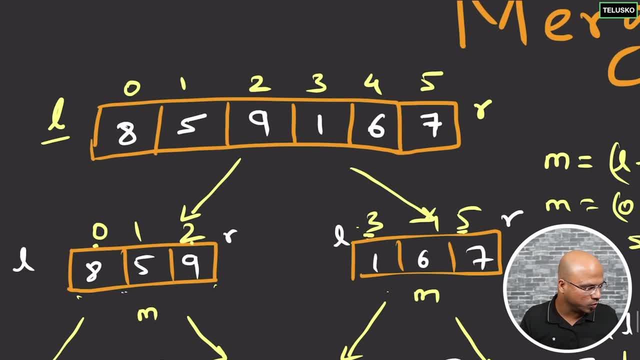 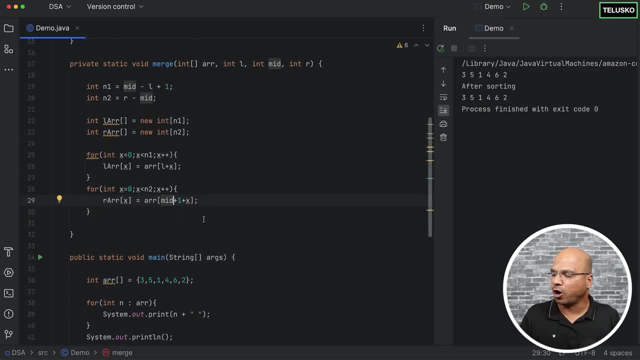 example, if you go up, the mid here was 2, but we started with 3, so you have to say 2 plus 1, mid plus 1, so that you will get 3. okay, so we copied was the next step, and now the actual work starts. 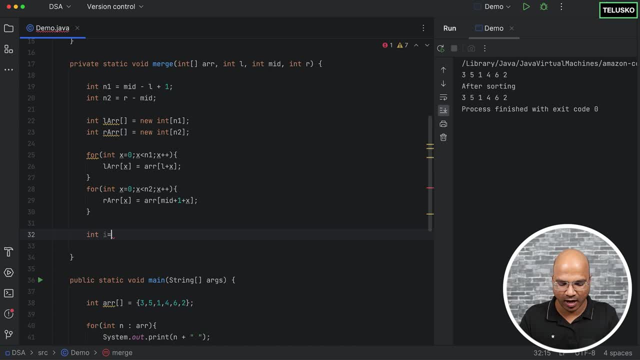 of merging and, already mentioned, we need two variables. one is i equal to 0. we also need j for the second array. so first array will be counted with i and second array will be handling will be handled by j. but we also need one more counter which will represent the main array, right, and this value will start with l. 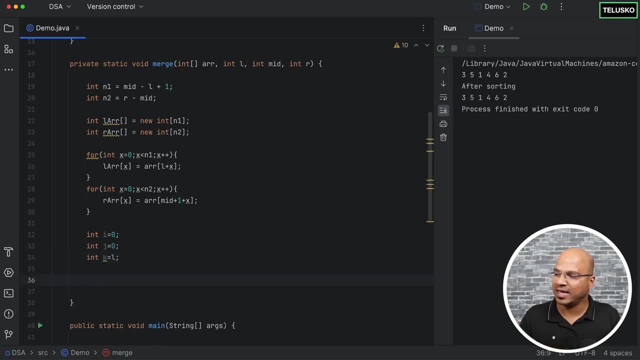 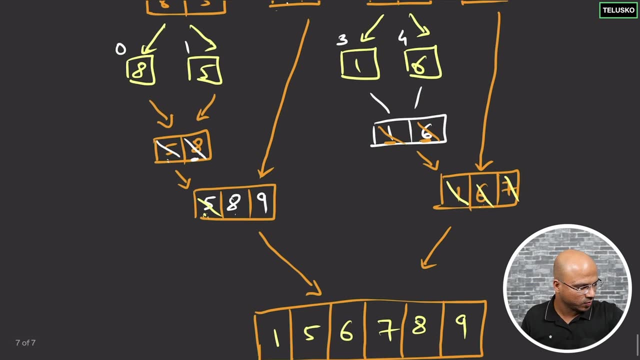 because you have to start from the left hand side. now, once we get these three values, let's start merging them. so we have to do multiple times right. when you say merge, you have to take my value from here. example: when we were doing this, we would compare the first two values, compare the next. 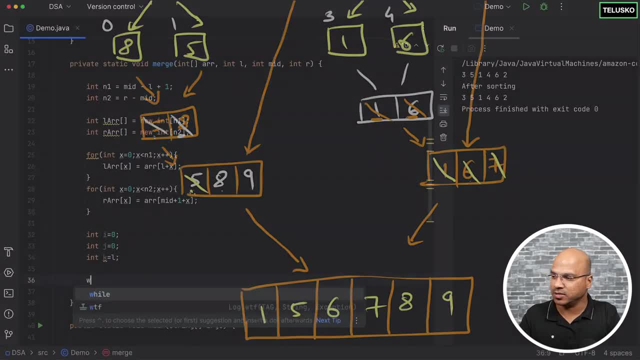 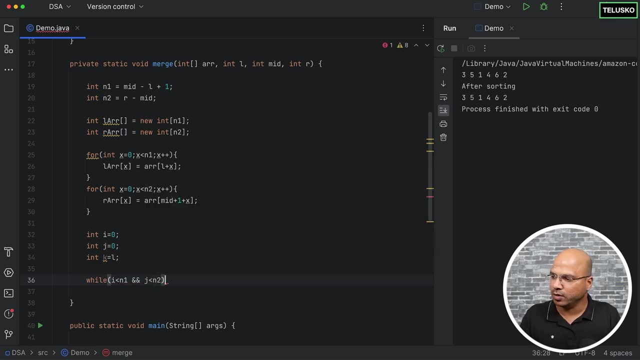 two values. that's how we were doing right. so when to end this, if your i value is less than n1, and not this hand and and j value is less than n2, we'll. we'll continue till this point. if they are not true, then we'll. 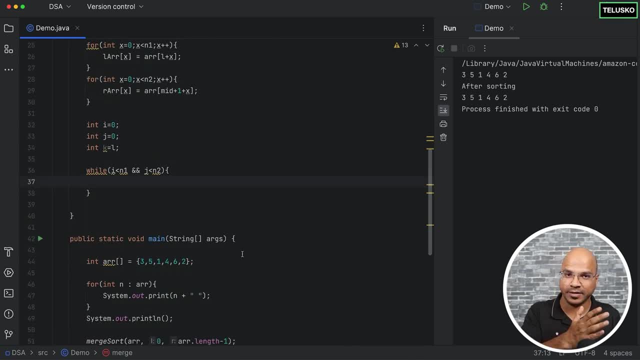 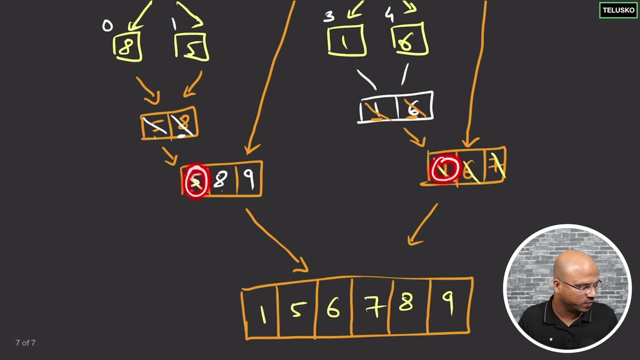 have to stop, because that means we have to, we have to reach the end. but now question arise: how will you merge? and that's where you have to start comparing values. now, when you say compare what it means? compare 5 and 1. so basically, the first element of this array and the first element of 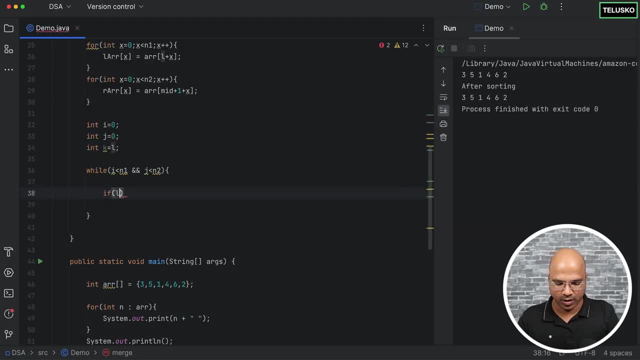 this array. let's compare them. how will you do that? so simply check if the l array of i- because that's what is representing the l array, which is the first element of this array, and the second element of this array is the i variable if it is less than, and we can also say: equal to what if they're equal. 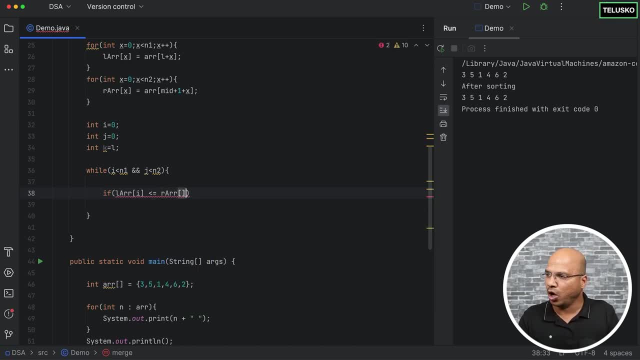 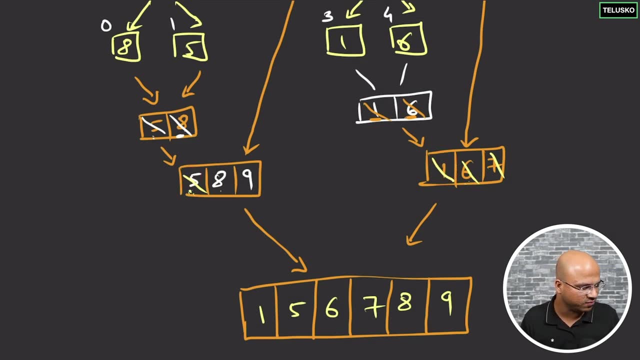 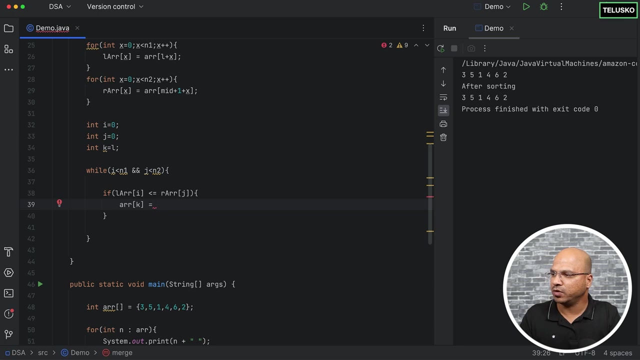 then we have to compare this with the r array of j. if the left one is smaller, in this case the r one is smaller, not the left one. but let's say, if the left, left one is smaller, in that case you will put that into the main array. so array k is equal to l array, not length l array of i. now, since we have 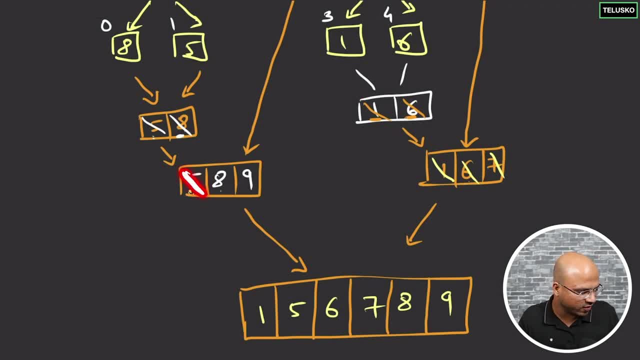 used. so let's say this was a smaller value, and once we have used this, we have to cancel this, right. i mean, this is done so we can shift our pointer to the next next element. how do you shift your not the pointer, but the reference? you will simply say i plus, plus here in this case. but what? 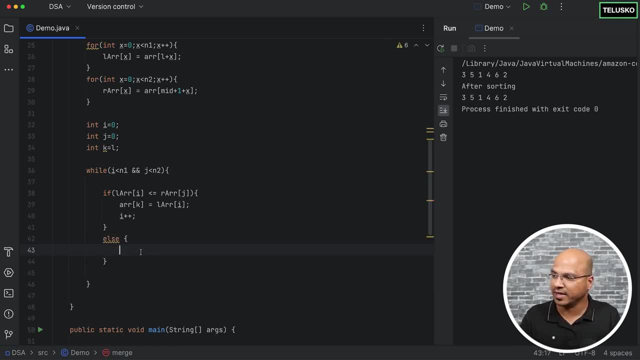 if it is not same or not, is what? if it is not true, in that case you will go to else part. you will do the same thing, but not with the left array. you will this time you will do with the right array and then the j variable and you will say j plus, plus. and every time you run this loop, because, see, 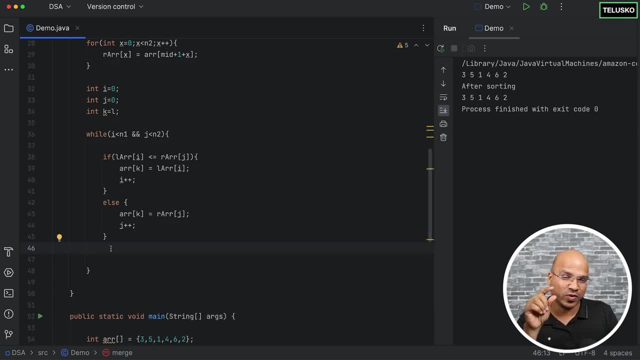 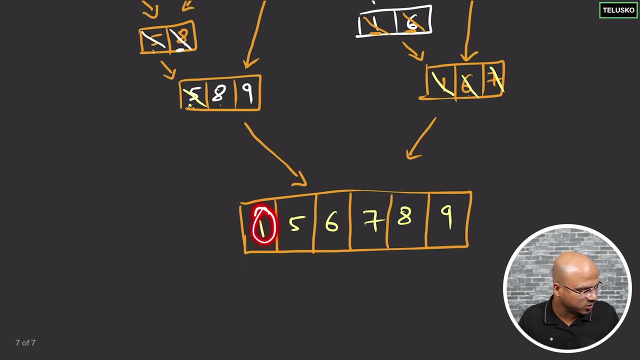 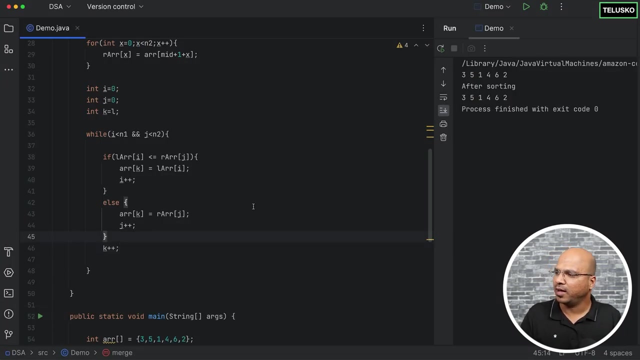 of this loop. basically, you will get the first value of the array, right main array. you will simply say k plus plus, because you have to also increment this. so once i is done, because k is here, once i, once i is done, you have to move k here. okay, and that's why we're doing k plus plus, and that's. 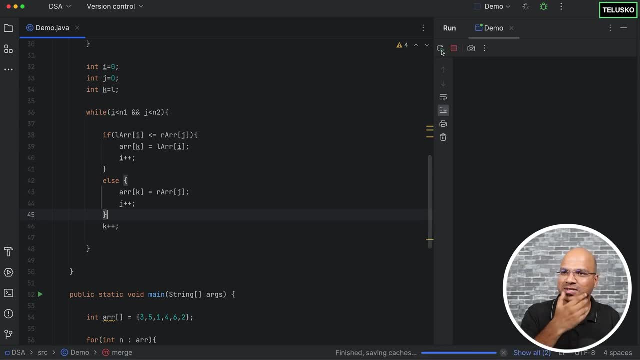 it. this is your merge sort. let's see if that works. let's refresh this. i'll just rerun. and we got an error. something went wrong. you can see everything was going well, but this four is not at the right place, so let's refresh this. and we got an error. something went wrong. you can see everything was. 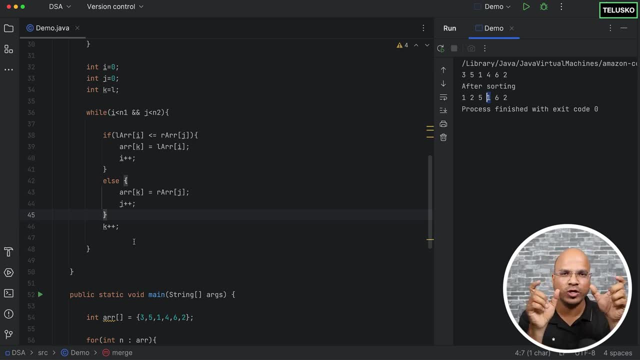 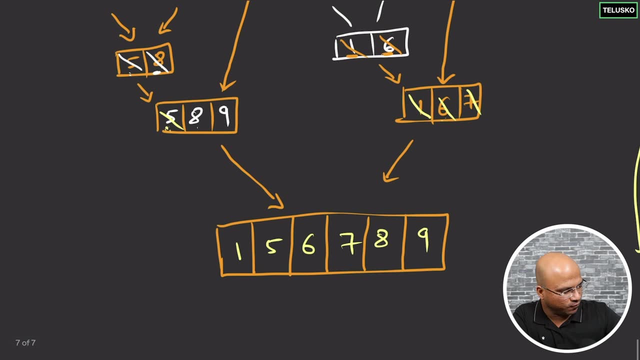 going well, but this four is not at the right place. we got one there because sometimes what may happen is when you're copying two arrays, what if the values are left in one of the array example. if you look at our example, when we were copying this, remember when we were completing the entire- 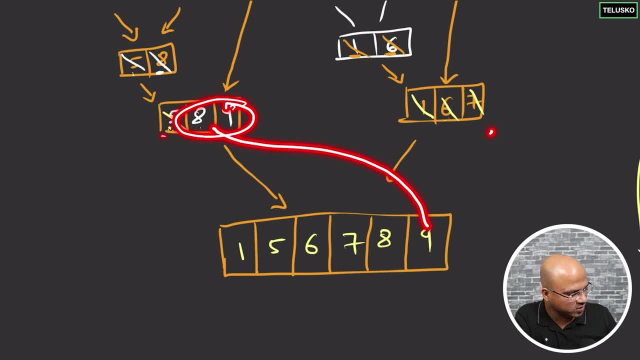 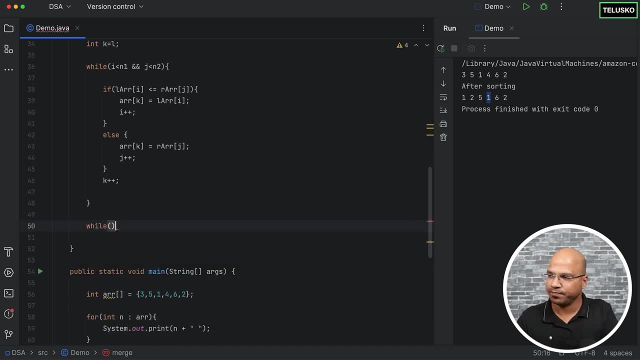 task. these two elements were remaining from the first array, which goes at the end, so that thing is not covered yet. so what you do is for the remaining elements of the particular array. you will again run a while loop here. so we'll say, if i is still not equal or still not less than 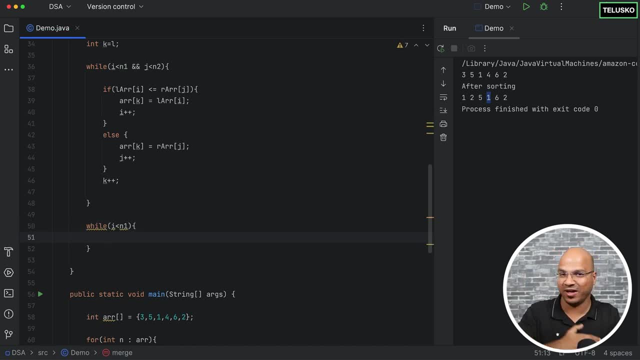 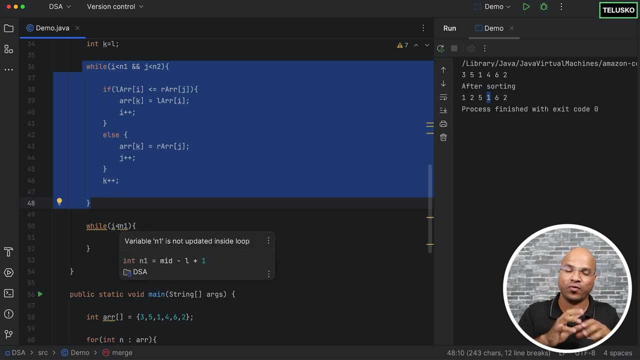 n1. you will simply copy the remaining elements, whatever is left, because after this loop at least one array will be ended. okay, so we have to work for the second of the remaining element of one of the array, maybe left inside or right inside. first we're trying to understand left inside. 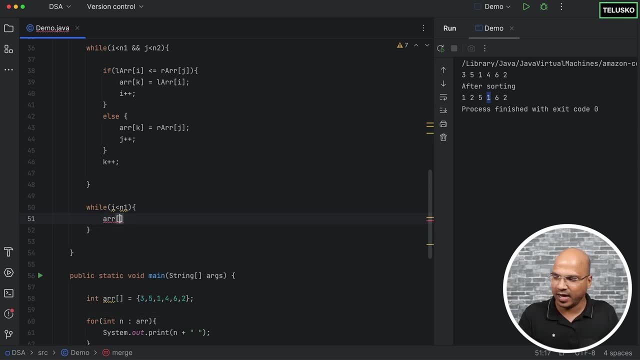 let's see what happens on the left inside. simply copy all the values so you will say: arr of k is equal to. we have to copy from the left array and let's use i here now. every time you do this you will increment both the elements, i and k, both. so this is what the left and right elements are. 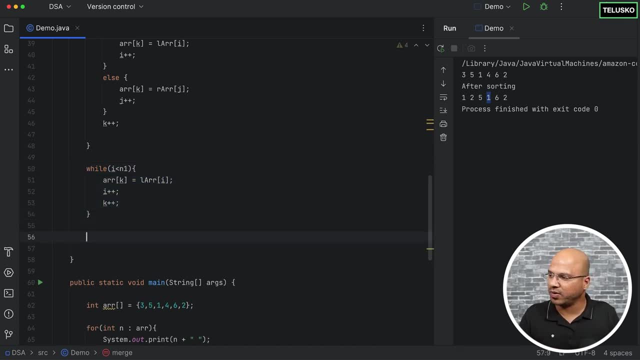 left inside, left out, left out values. the same thing should be done for the right hand side. so this time i will say j is less than n2. in that case you will copy, but not from the right left hand side. you will do it from the right hand side. the variable is j and the increment you will do. 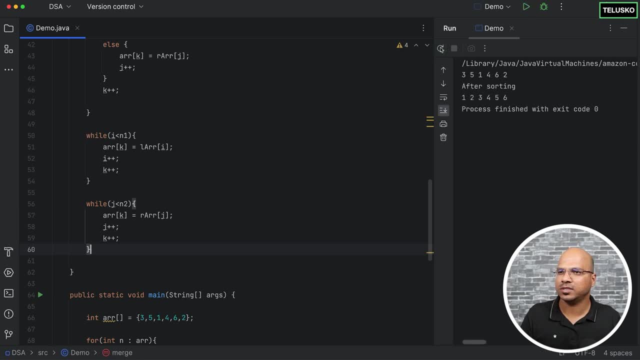 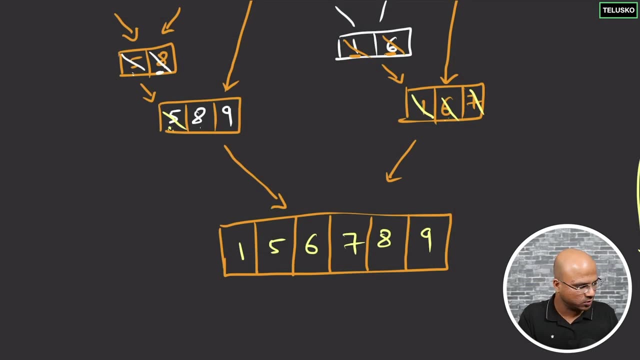 for j plus plus. okay, and let's run this and you can see. now it is sorted. and now it doesn't matter what values you have. let's say, let's take the values which we have returned on the board, which was eight. what was the value? eight, five, nine, one, six, seven. 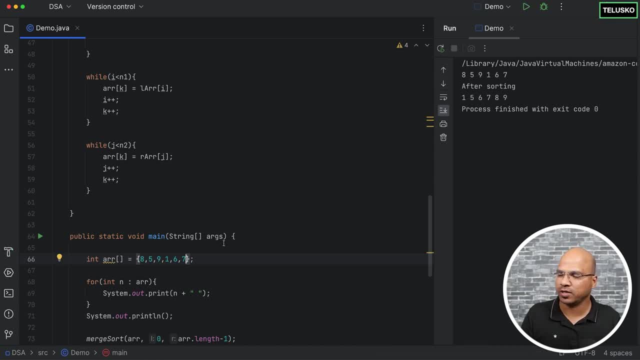 and if you run this you can see we got sorted values. let's add some more values here, just to remove the confusion with different values. let's say one, one one. this is fifty seven. and now let's see six, seven, eight, nine, fifty seven, seventy five. one, one one. so this is your merge sort, so the 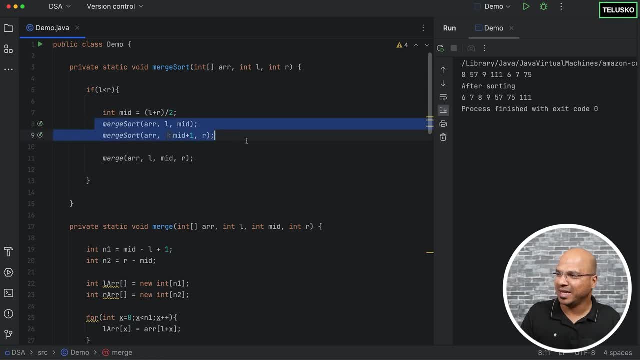 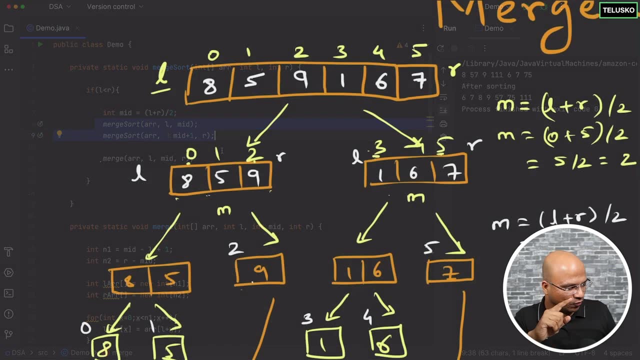 steps. basically, you have to first do the breakdown of, you have to break the array down into small chunks, and then you have to also merge them. the only thing you have to remember is when we were drawing this, we have to add a new array and we have to add a new array and we have to add a new array. 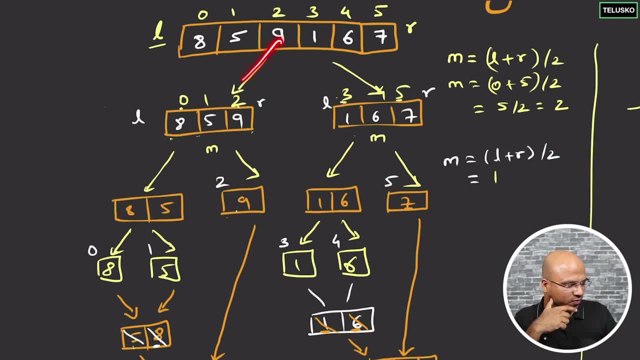 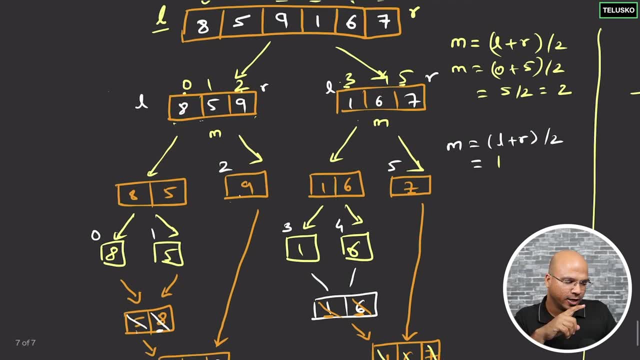 we were going in two sections, right, something like this. we were saying: okay, we will create two different section and then first section will break into two parts and second section will break into two parts. no, that's not how it is working. if you observe what it will do, is it? 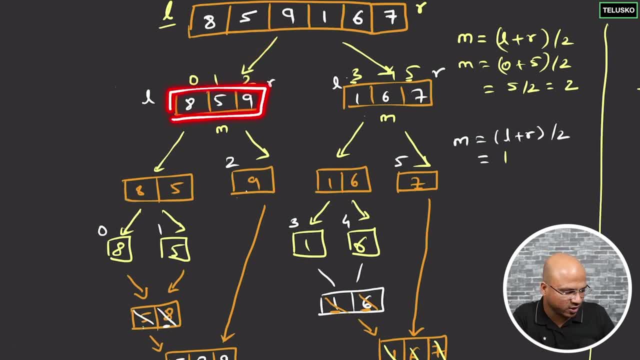 will break down the entire section into two parts. yes, but then first only you will get the first part, then you, you're not going to the second part. okay, you're not looking at here. you, this is not there yet, you're still into the first part. then this will divide into a section. you will get this. 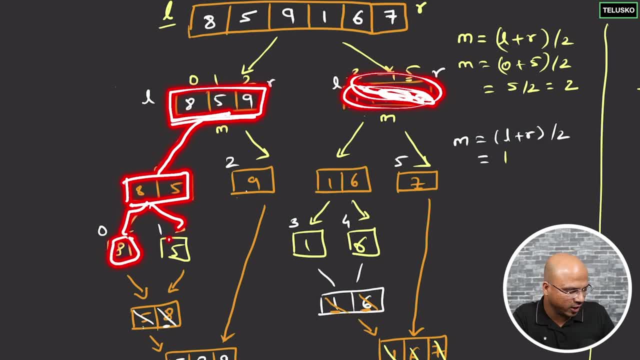 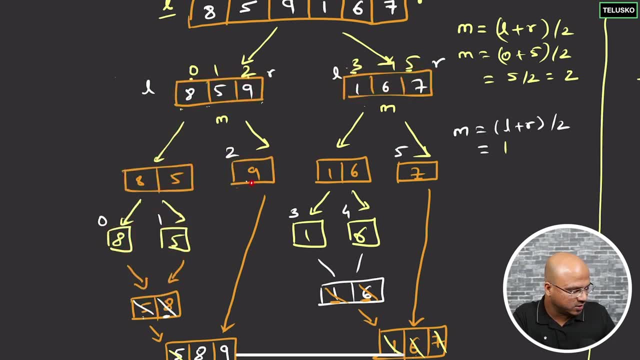 eight five. then you're dividing into two sections, which you will get eight five and then you will. then you will start breaking down the second part, which is nine. okay, nine was still not there. then once this is also merged, once you get this, it will start working on the next part. then it will work on. 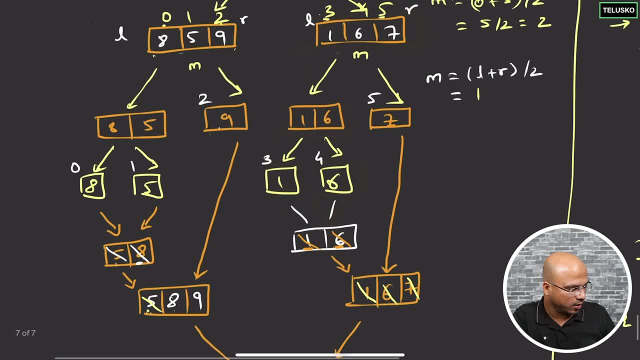 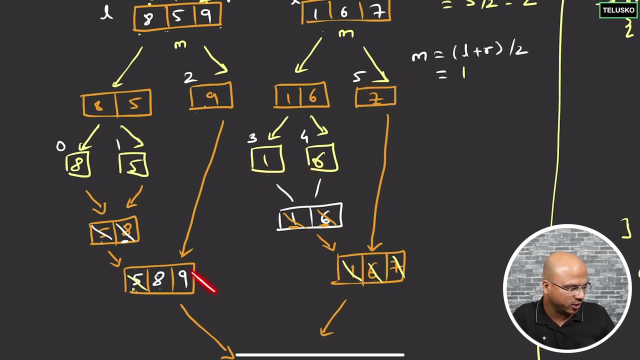 this. it will work on this, this merge and merge. i mean, sorry, break down, then you get seven, then you merge this two and then, once you have merged, then it will go for this next two. so it's not exactly breaking down the entire section. equally, it's basically going from left to right. so yeah, that's. 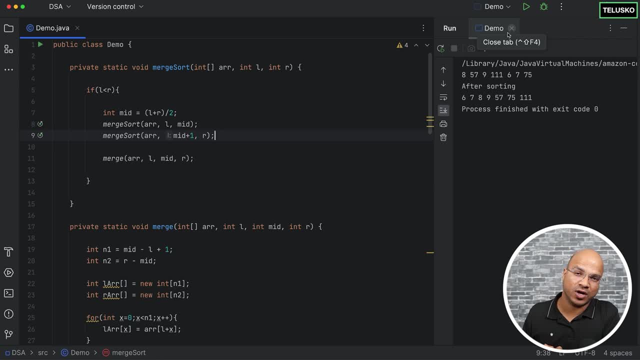 how things are working in the next section. so yeah, that's how things are working in the next section. out and this is your merge sort with the help of java code, and i hope this makes sense. let me know in the comment section. see you in the next video. 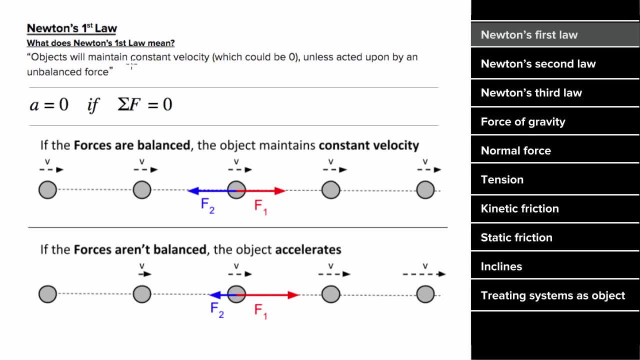 What's Newton's first law say? Newton's first law states that objects don't change their velocity unless there's an unbalanced force. So if there is no force on an object or the forces are balanced, then the object will continue moving with a constant velocity. Or if it was at rest, 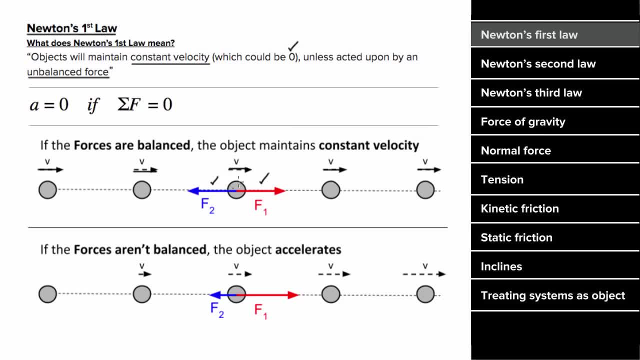 it'll continue sitting at rest. In other words, there doesn't have to be a net force for something to have motion, There only has to be a net force for something to have acceleration. And it's really important to note that Newton's first law does not only apply to single objects, it applies to